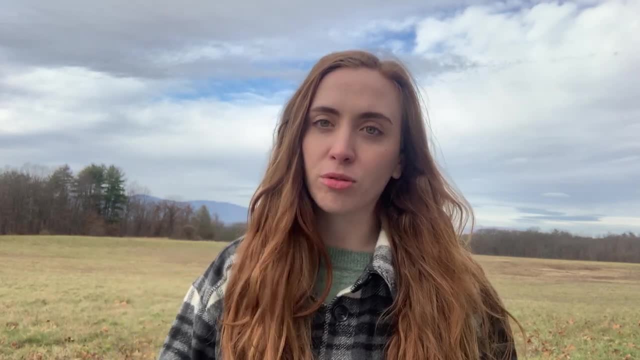 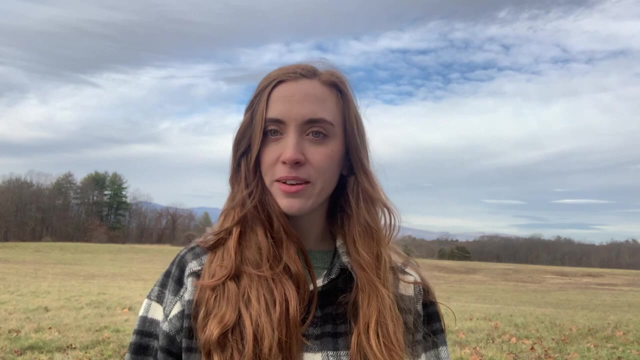 to understand geologic time if you're looking at it through that lens. So how do we understand geologic time? How do we know about all of this stuff that happened in earth's history when we weren't here for most of it? How do we even know that earth is 4.6 billion years old? to begin with, 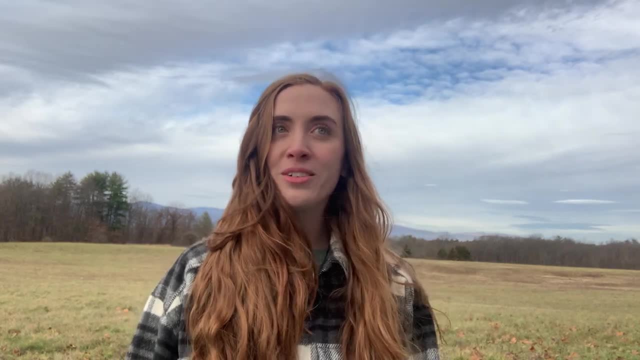 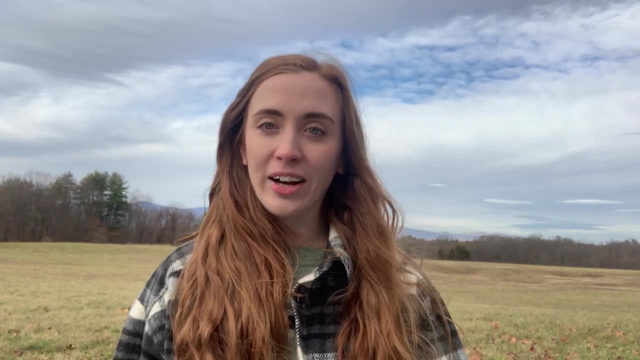 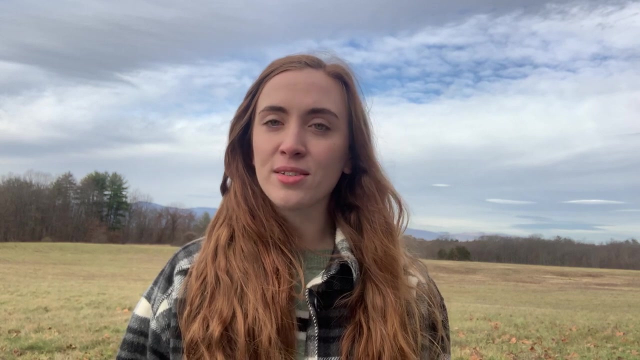 This is because of the rock record. Rocks are so interesting, and this is one of the many reasons why Think of the rock record as a global library of books, many of which haven't been read yet. There's all these books waiting to be read, and they tell us so many stories about earth's history. 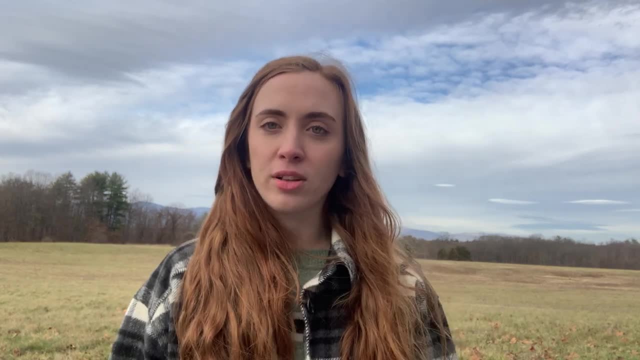 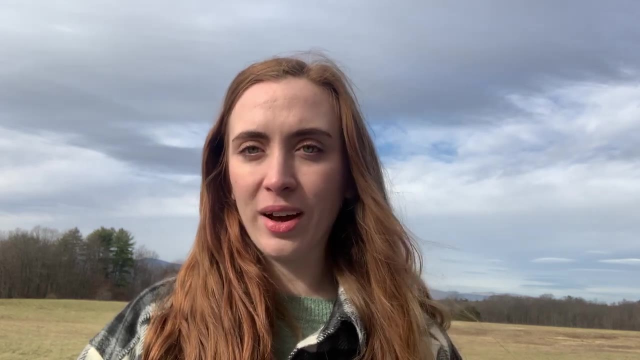 and all these events that happened geologically and biologically throughout time. So what do we look at in the rock record in this giant library to figure out what the heck happened before we were here? The two things we talk about are relative dating. 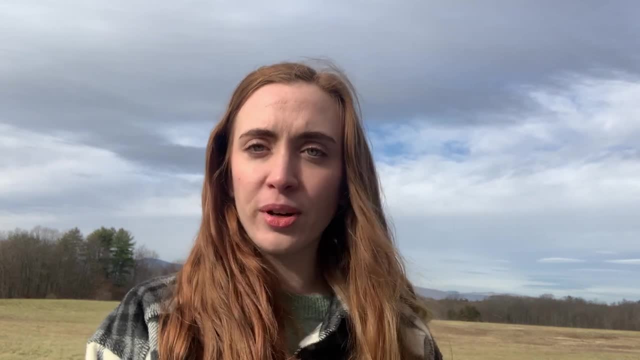 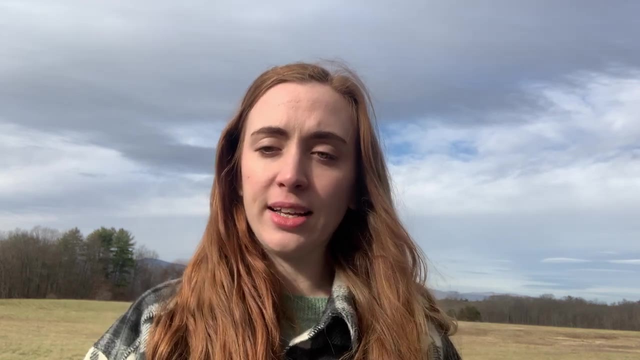 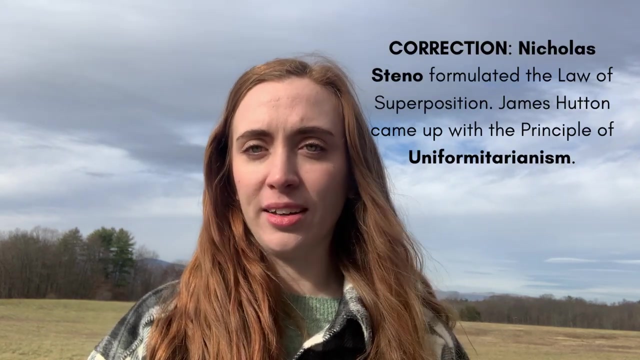 and absolute dating. Before the 1900s, before the discovery of radioactive materials, we used relative dating. Relative dating is taking the strata, the rock layers, and comparing them to each other to figure out the sequence of events. Someone named James Hutton came up with the. 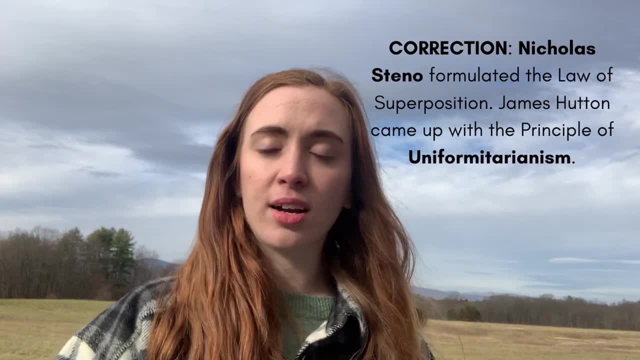 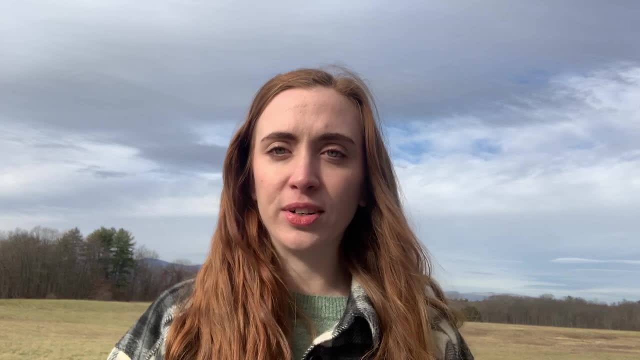 principle of superposition, and this states that the oldest rock is on the bottom and the youngest rock is on the top. This is something that you subconsciously think about every day of your life. Take your house, for example. In your house there's furniture, But before you could get the 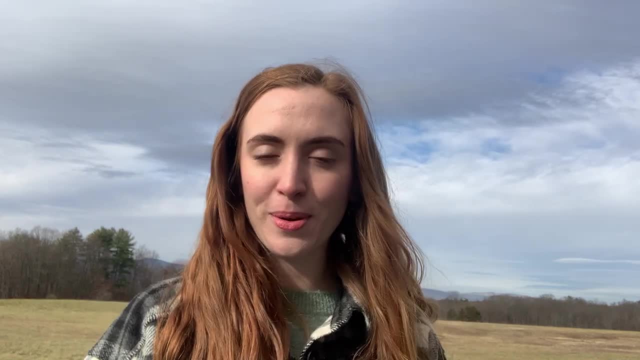 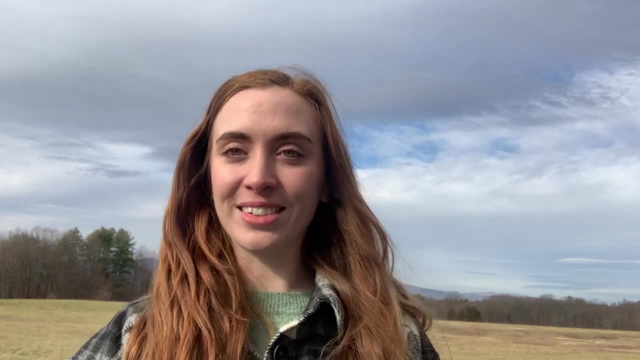 furniture in there. the house had to be built, So the foundation was built. the frame, the sheet rock, I don't really know, I'm not. I'm not a house builder, But you know what I mean. All that stuff happened and then you put the furniture inside. Then you put: 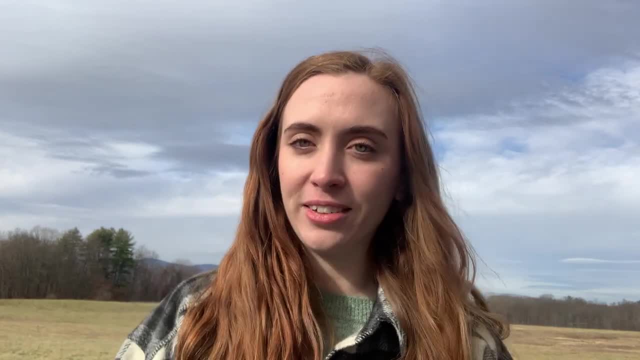 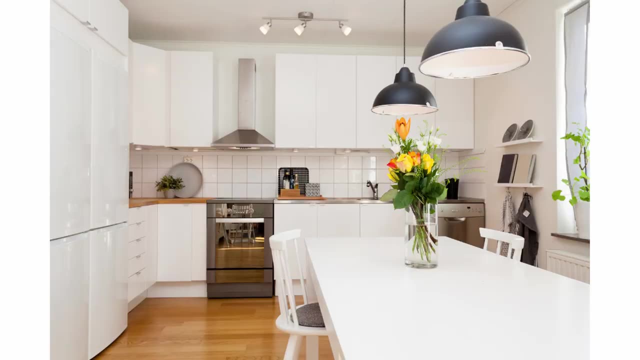 all the decorations up and you put your sheets on your bed, then your blankets and the pillows. You can tell by walking into someone's house, unless they're very strange. you know the order in which these things occurred. You don't know the exact date and time that these 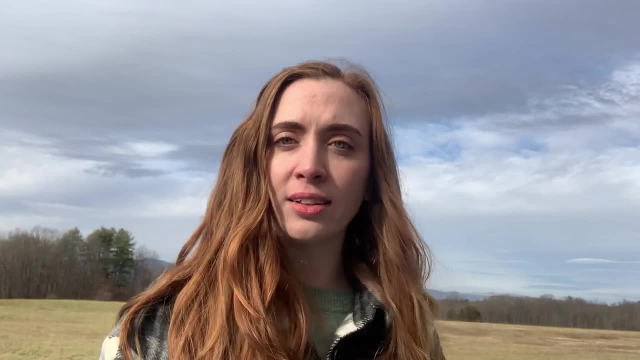 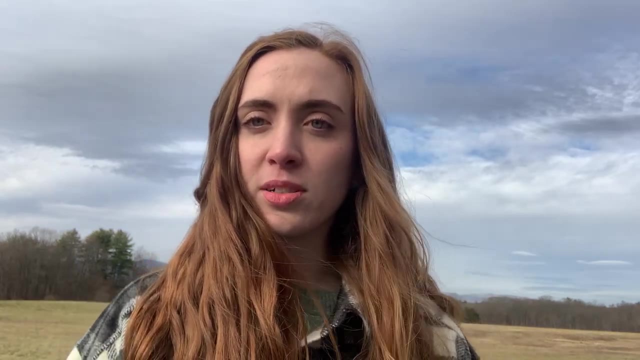 things happened. but you know the order. You could go through and write a list. This thing was put here first and then this thing. This is kind of like the concept of relative dating. So really important principle to talk about when we are talking about relative dating is the principle. 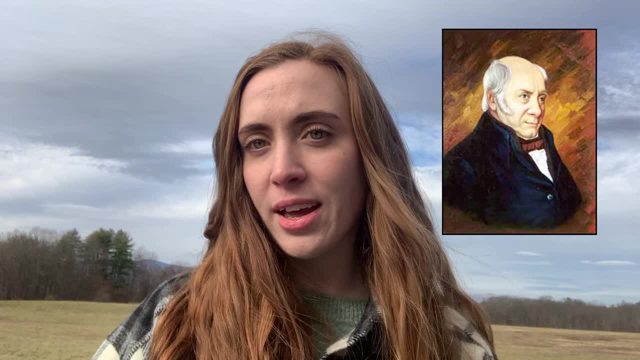 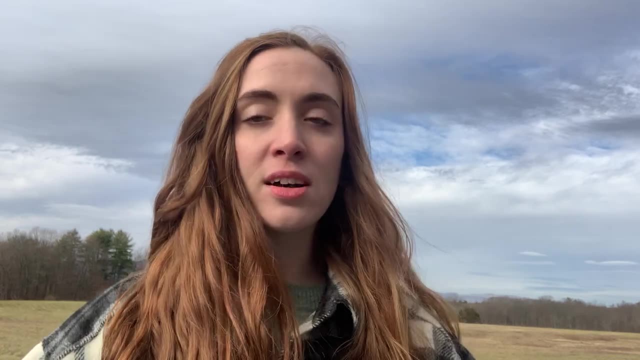 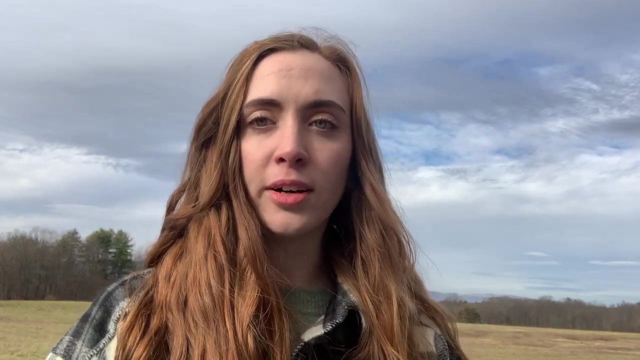 of final succession. William Smith was an English engineer and surveyor and he was looking at the rocks and the fossils and he understood that fossils go through this sequence of events. You can look at them in the rocks and you can say this fossil is older than that one, because this one 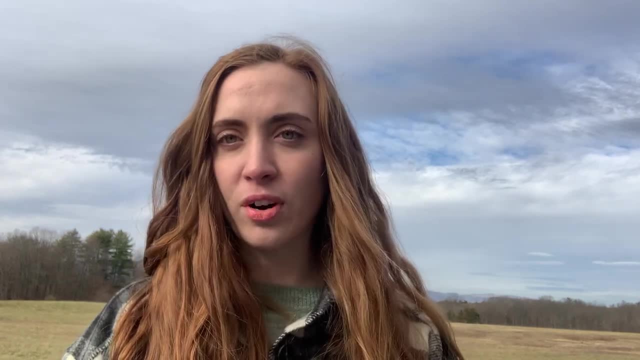 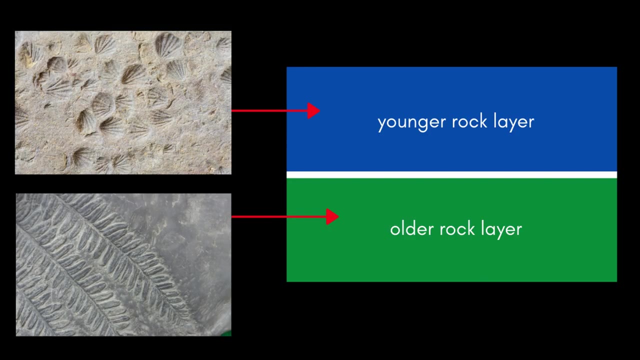 doesn't have legs and this one does. He was looking at all these different rock layers, and the rock layers are completely different from one another. Some of them didn't even have fossils. This is extremely important to relative dating and this was the main way that we were able to sequence. 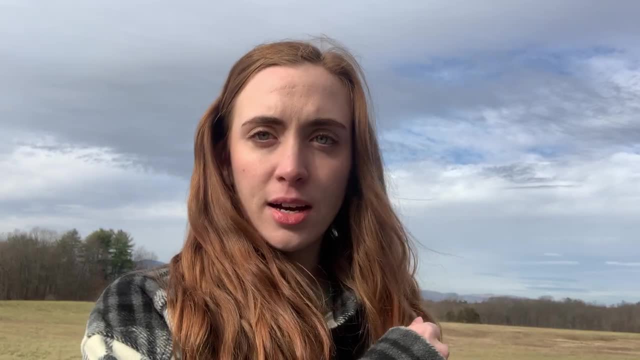 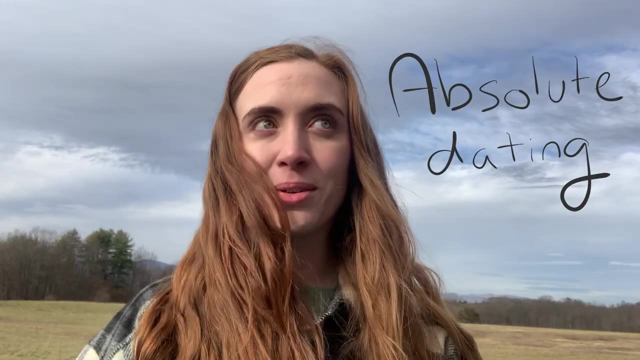 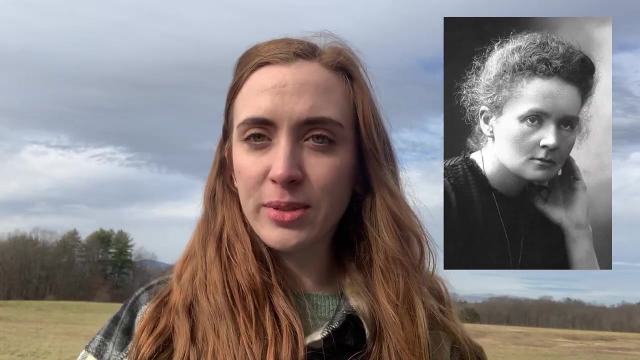 rocks and rock formation events before the discovery of radioactive materials. That brings us to absolute dating. So absolute dating was made possible by Marie Curie, who in the early 1900s discovered radioactive materials, specifically radium. After this discovery there was a huge 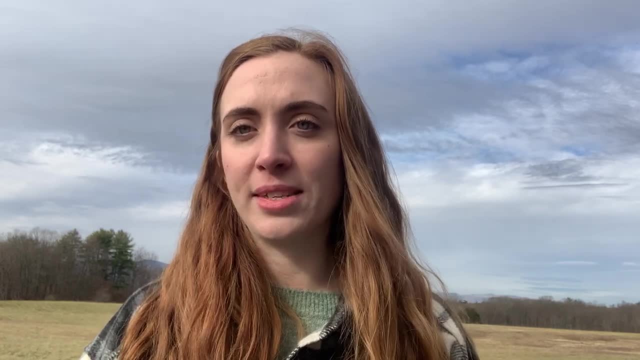 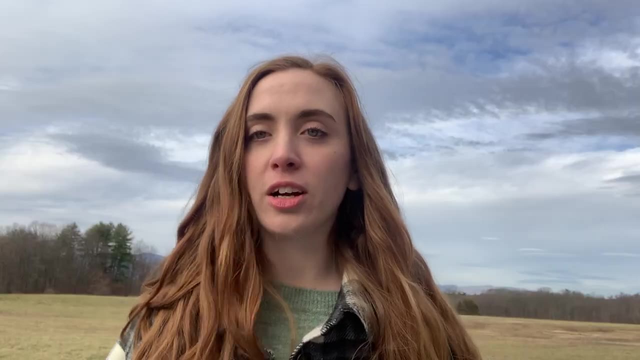 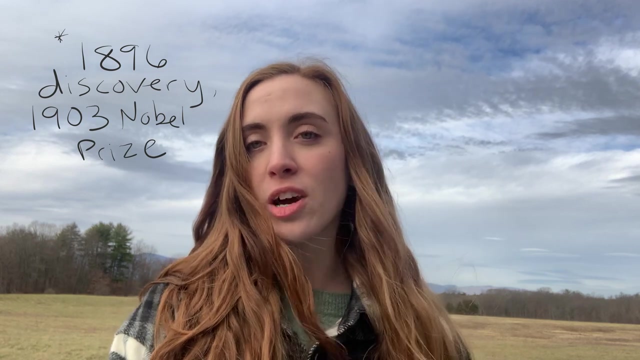 change in how geologists and scientists were able to assign dates to things. We were able to take these radioactive materials and calculate how old they are. Marie Curie's groundbreaking discovery of radium in the early 1900s jump-started a new way that geologists were able to organize. 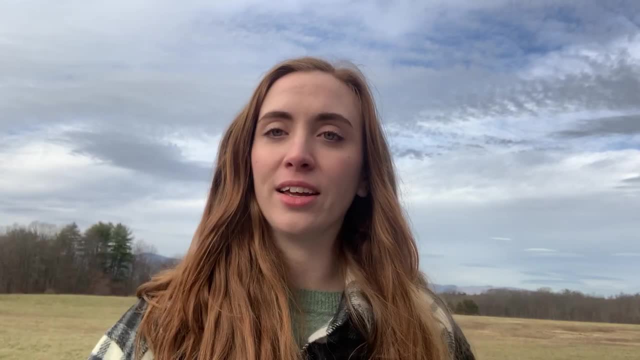 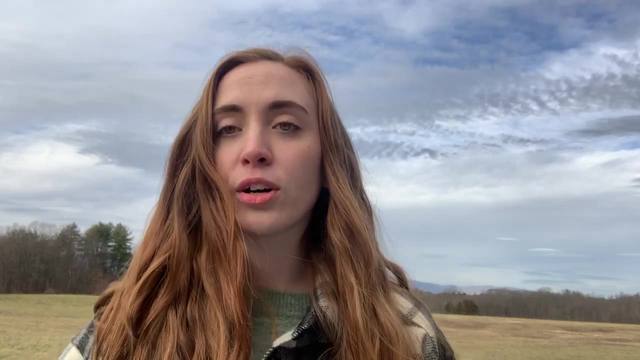 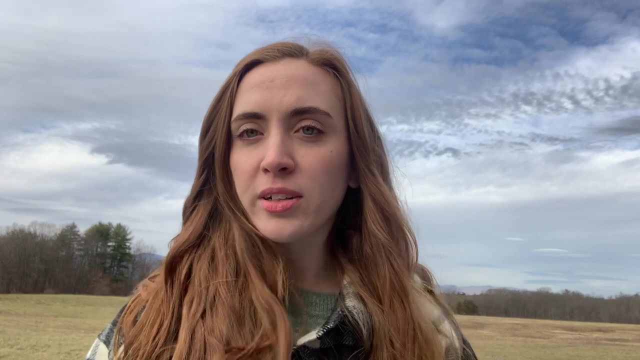 the geologic time scale. We still use relative dating when we can't use absolute dating, but absolute dating has become the main source of figuring out the age of a rock. It also confirms the relative ages of things that we figured out before absolute dating was a thing. A couple examples of elements commonly used in radiometric dating are uranium-238,. uranium-235,, rubidium-87,, potassium-40,, samarium-147, and carbon-14.. Carbon-14 is a mineral that contains uranium-238, uranium-235, and uranium-235.. Uranium-238 and uranium-235 are. 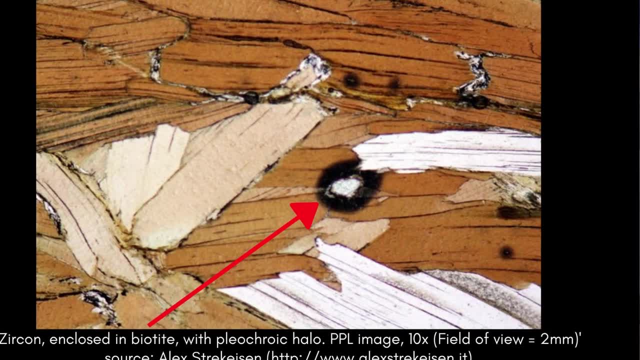 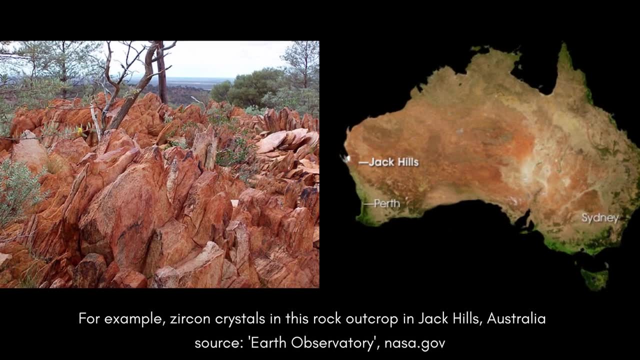 common in zircon crystals. Zircon is a mineral that is actually extremely old, and it's found in some of the oldest rocks on the planet. Other minerals that have uranium in them are biotite, muscovite amphibole and potassium feldspar. 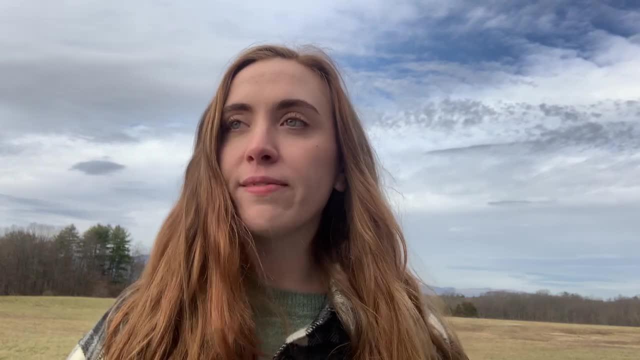 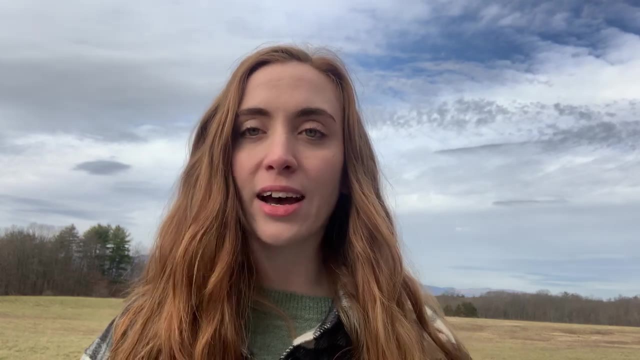 So this brings us back to that house analogy and the furniture. If I was able to go into your house and put post-it notes all over every single item and say exactly the date and time that you put them there, it only confirms the relative ages I assigned to them before, but it gives me more. 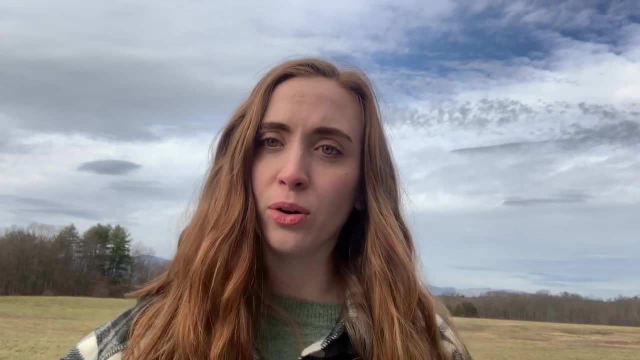 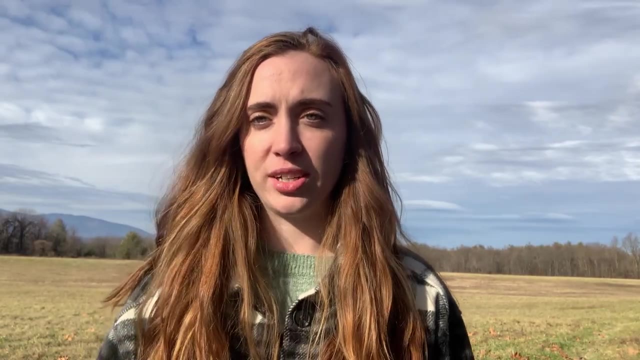 information more than I had before when I was just putting them in order from oldest to youngest Just got very sunny. So as you go and start learning about rocks and rock formations, you'll realize that they are not the same as they used to be. They're not the same as they used to be. 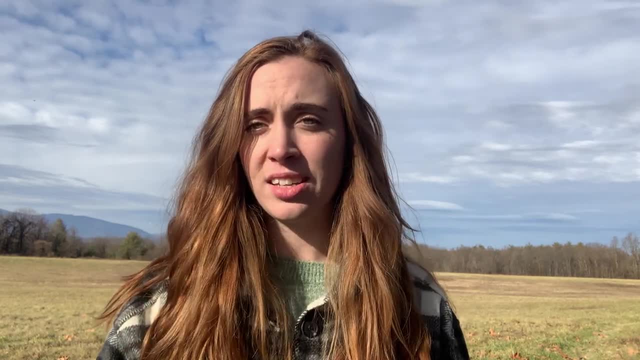 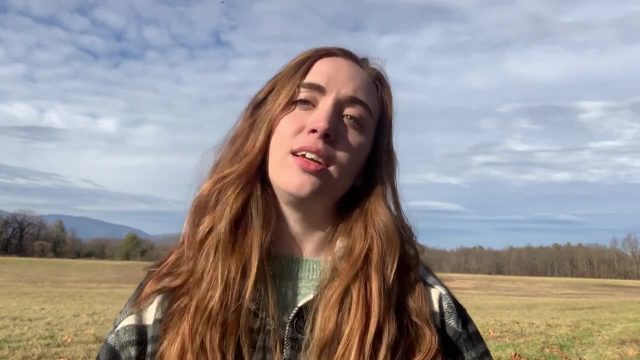 They occur in thousands to millions of years, to even billions of years, And this is really hard for the human brain to understand at first. We're used to thinking in days, weeks, months, years, decades, So how can we understand millions of years and billions of years? How big is a? 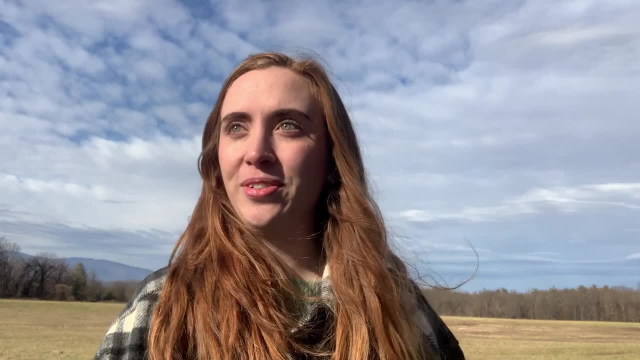 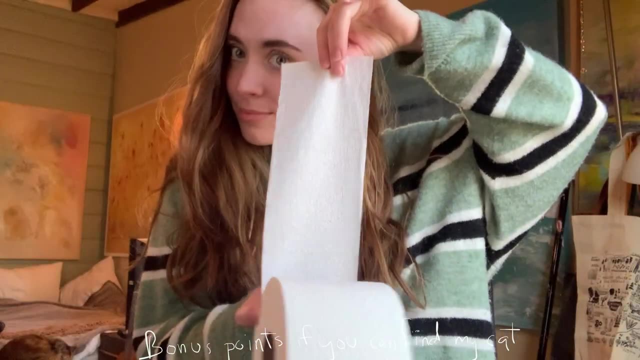 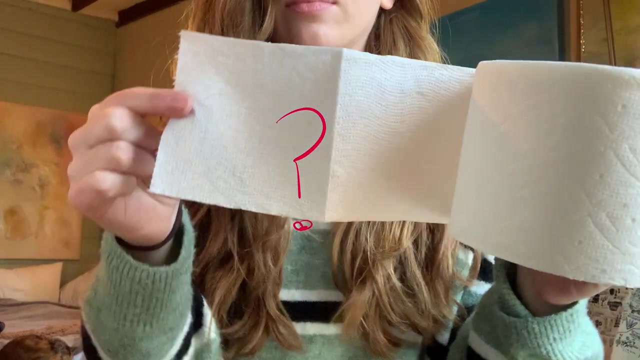 billion. So I thought a nice little example to use to figure out how big a billion really is is toilet paper. So if you take one sheet of toilet paper and you say this is 4,000 years, So if each sheet is 4,000 years, how many sheets of toilet paper would it take to represent one billion years? 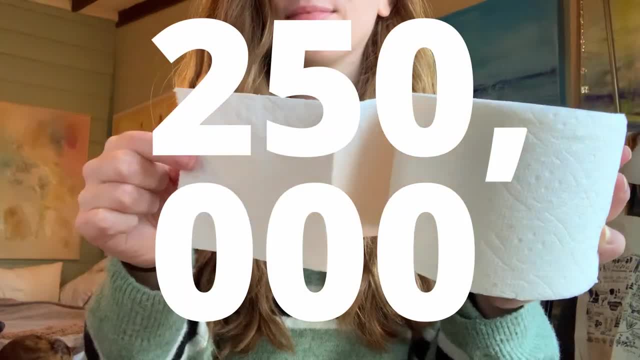 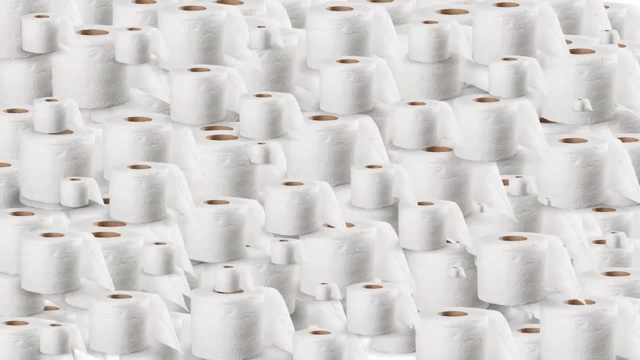 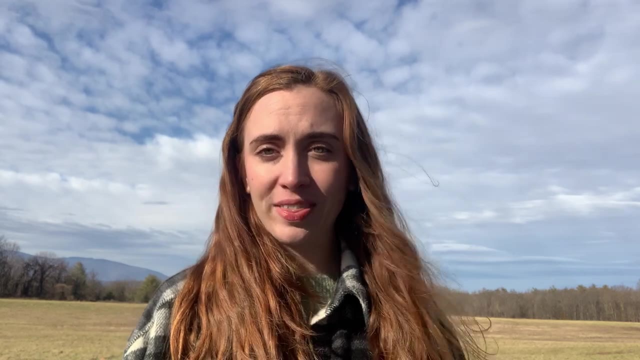 This would take 250,000 sheets of toilet paper just to represent one billion years. I think there's about a thousand sheets in one roll, So you would need about 250 rolls of toilet paper. to show a billion years. For the entirety of earth's history, you would need about 1,150. 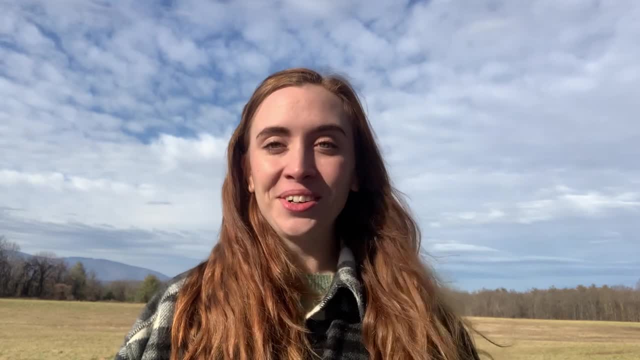 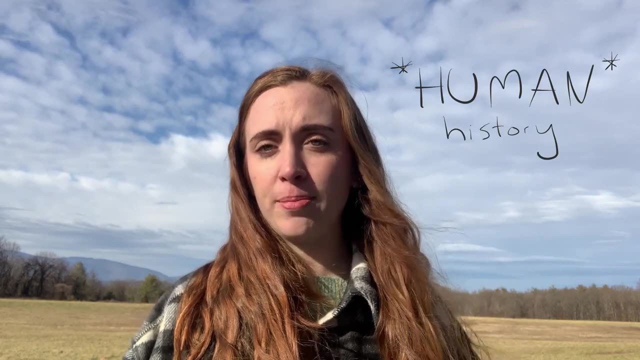 rolls of toilet paper. That's 4.6 billion years. That's a lot of toilet paper. There probably isn't that much at the store right now because of COVID And the entirety of earth's history is only about 2 million years and that's about 500 sheets of toilet paper. That's not even a whole. 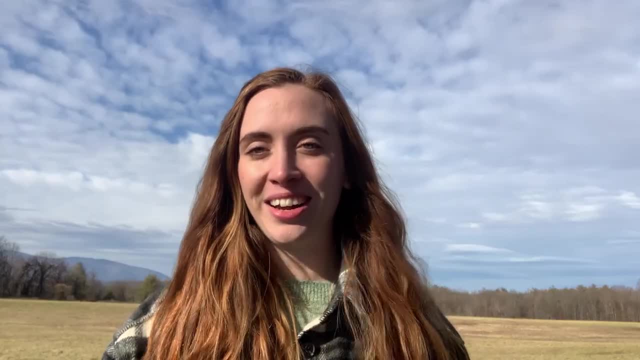 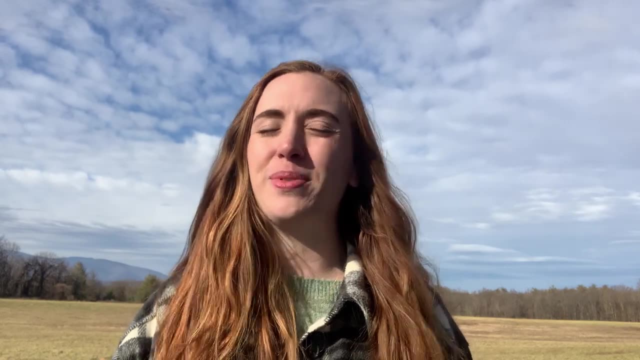 roll of toilet paper. So I think that's a pretty good analogy of trying to understand what one billion years actually looks like. I don't think that's something that any of us as humans are ever going to truly be able to understand, because it's just not something our brains are meant. to understand The hierarchy, like I said, starts out with eons as the biggest category. There are major eons in earth's history on the time scale, and those are the Hadean, Archean, Proterozoic and Phanerozoic. The Phanerozoic is split up into eras. These eras are Paleozoic, Mesozoic. and Cenozoic. Paleozoic was marked by a big explosion of life of all different species. This is called the Cambrian explosion. This happened at the beginning of the Paleozoic. Mesozoic was marked by dinosaurs, whales and birds, as well as lots of different plant life, Cenozoic or recent life. 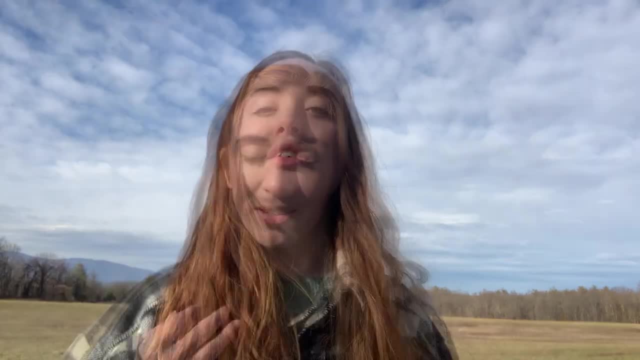 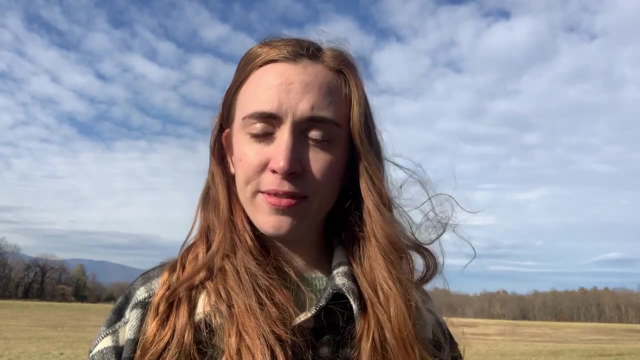 is marked by the dominance of mammals on planet earth. So the last thing I'm going to talk about is mass extinctions. Not only is the time scale organized by the appearance of life, such as the appearance of the first single-celled organisms or the first multicellular organisms, but it is marked by the disappearance of life, known as mass extinctions. A mass extinction is marked by about 5% or more loss of species all over the planet in a short amount of geologic time. There were five extinctions. The first one was about 443.8 million years ago. The second one was 358.9. million years ago. The third one was the biggest one at the end of the Permian, about 251.9 million years ago, And it actually marked the transition from the Paleozoic era into the Mesozoic era Era Without this extinction. it might not have been possible for dinosaurs to evolve and take over the planet. The fourth one was at the end of the Triassic, about 201.3 million years ago, And then the last one was the end of the Cretaceous, with the extinction of the dinosaurs. like I mentioned, That one was about 66 million. 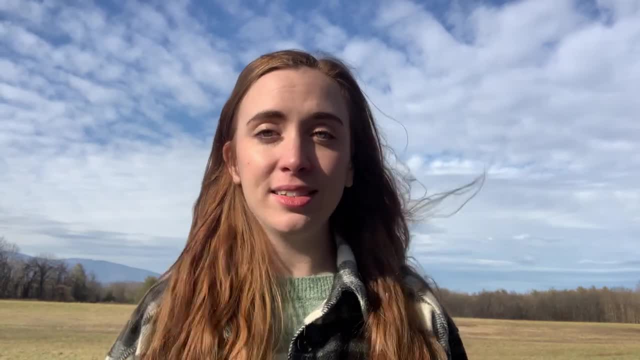 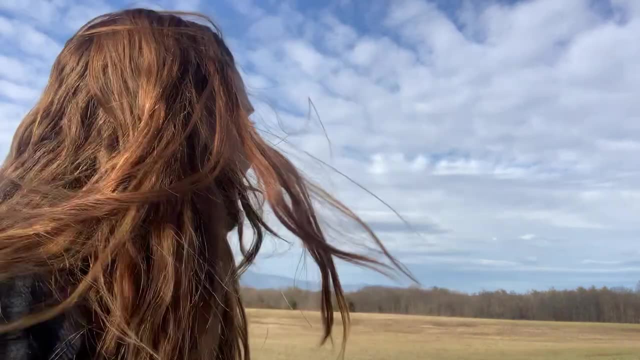 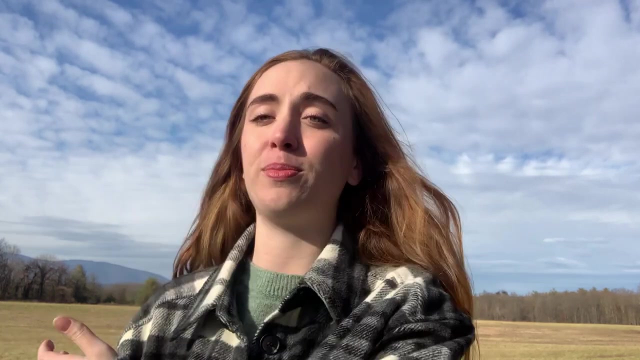 years ago. When you think about rocks, you may not think of living things, but living things are very important to the rock record and it's really windy. The time scale is continuously being improved upon, New discoveries are being made, So who knows, maybe in the next 10 years or 100 years there. 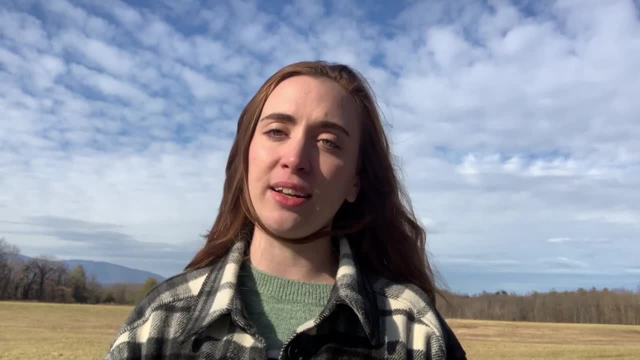 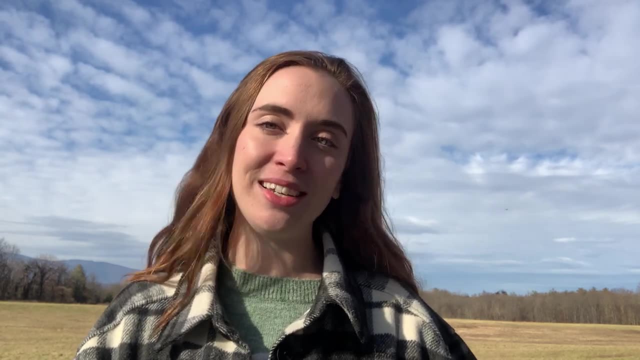 might be some crazy discovery that completely changes our understanding of the geologic time scale and Earth's history, But as of right now, this is what we understand about it, given what we've seen in the rock record. So that's pretty much it. I hope that this gave. 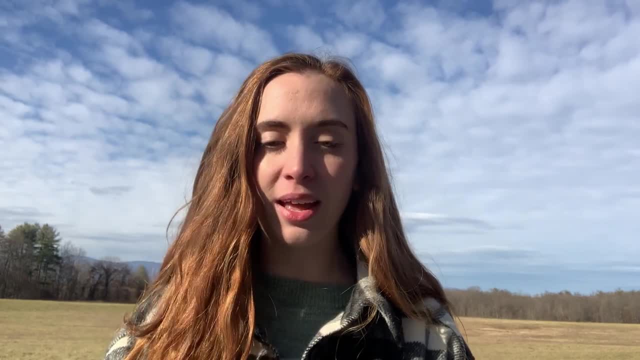 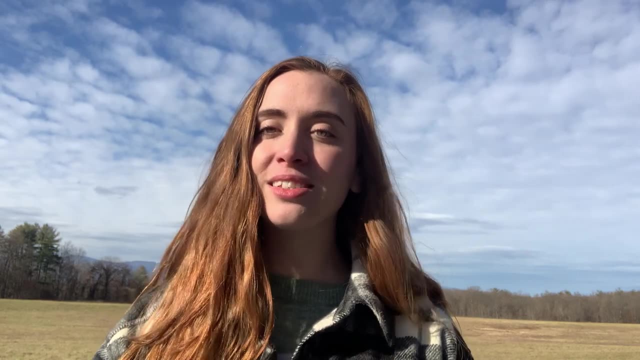 you a pretty good understanding of what geologic time is about and why it's important to know about it. If you like this video, feel free to give it a thumbs up and subscribe to my channel If you want to see more videos about geology and geology-related topics. Thanks for watching. 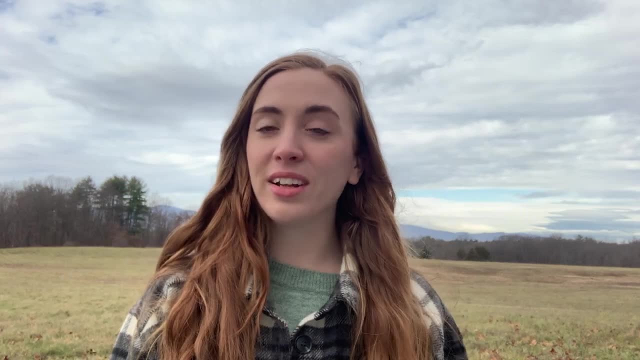 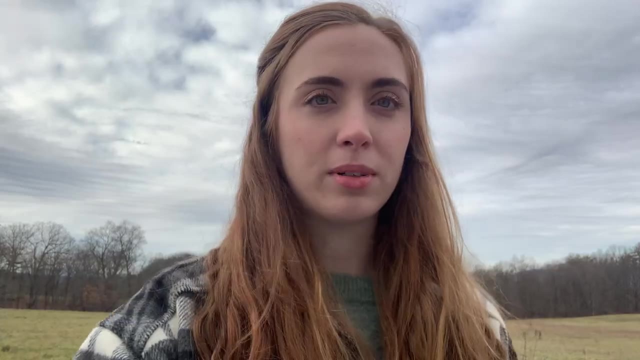 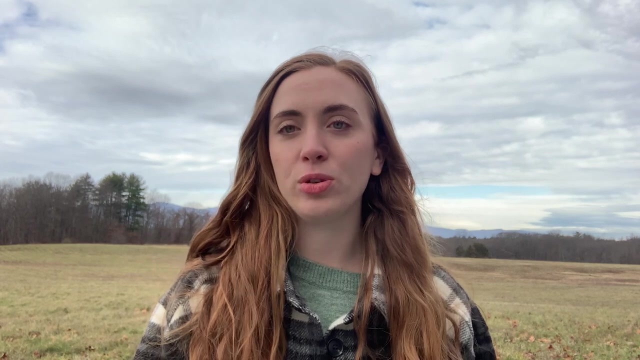 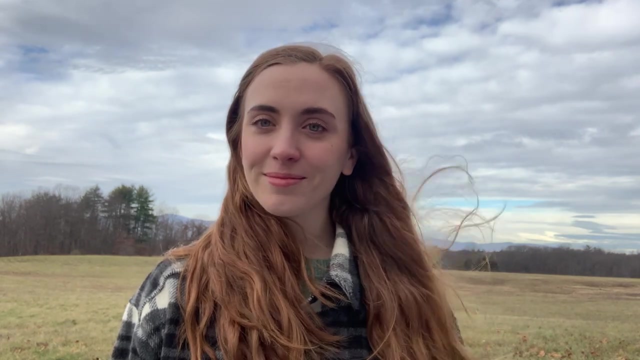 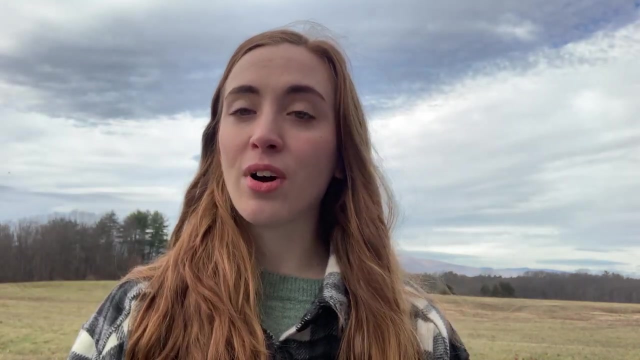 It's a bus Categorizing things when we don't really understand them at first and putting them into categories 4.6 billion years ago- Big breeze. Why would we need The geologic time scale? was made because of rocks. Those birds were just moving in a really cool way. Made because the 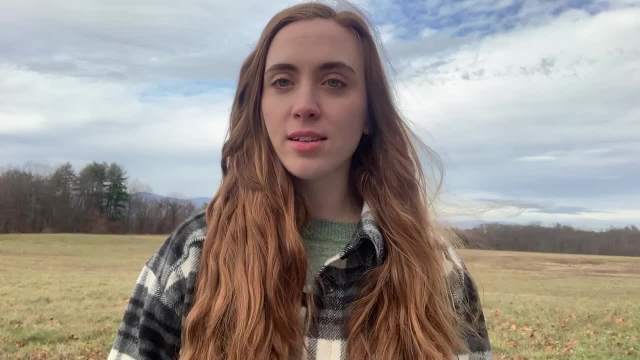 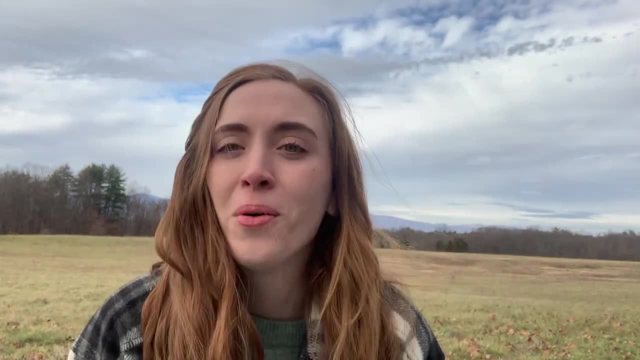 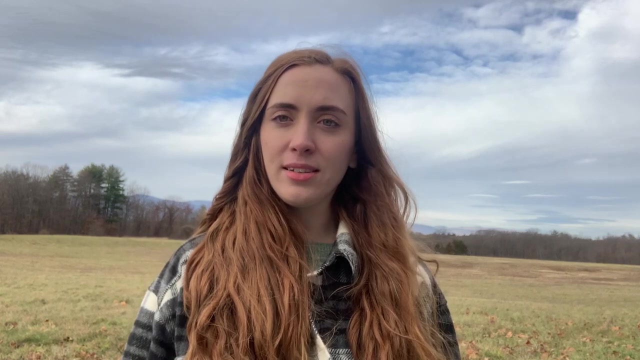 So why should you care about the geologic Rocks form in Wash? Oh my god, I'm cold. 4.6 billion, Most of the time, The 4.6 years of history. that Cold, Someone needs James. 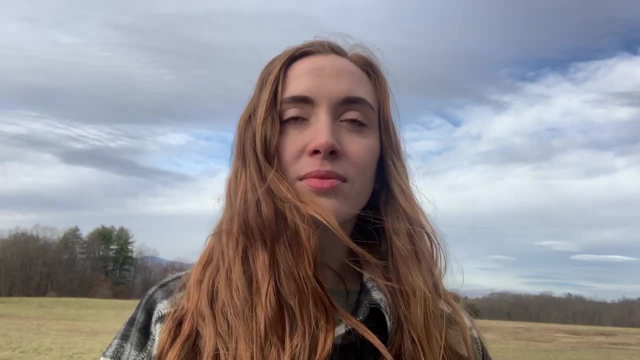 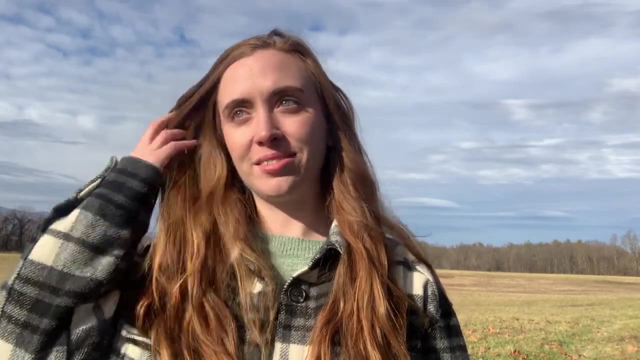 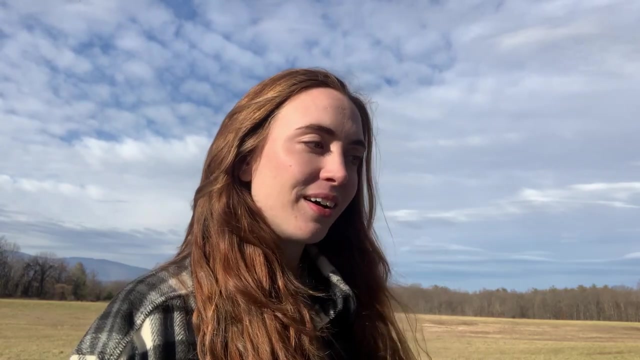 Huth Superposition What I would have written down about. We're not used to thinking in this time. Even If you had, I thought of a nice little analogy.